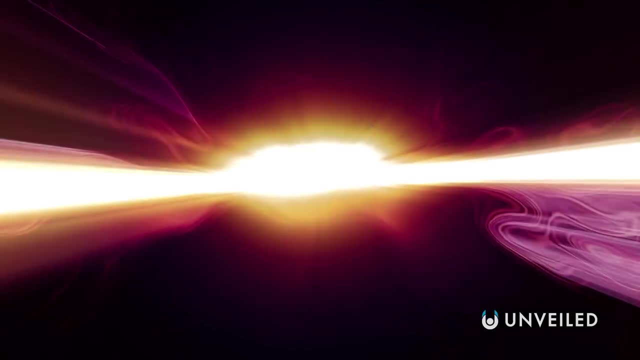 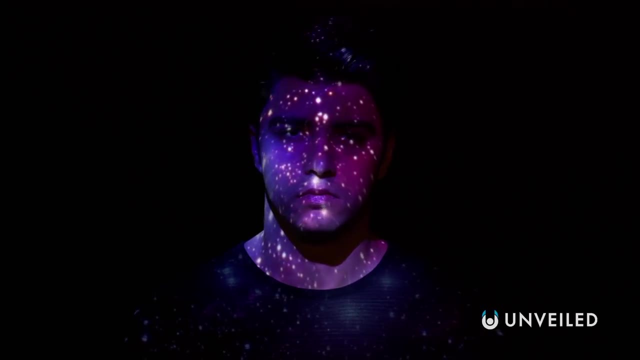 more than one EEV is packing a truly staggering amount of energy, Seeing as we're getting hit by cosmic rays all the time, though, what is it that makes the one sighted in Utah in 1991 so special? Well, to this day, the Oh My God particle remains the highest. 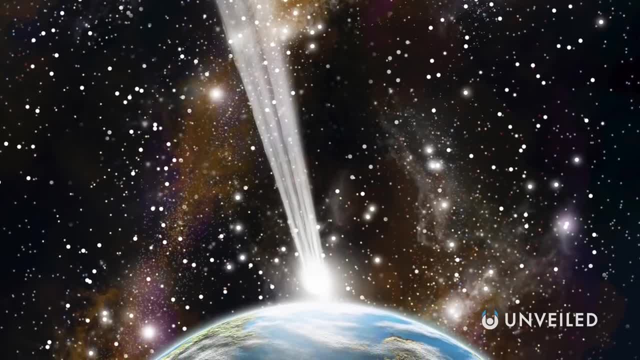 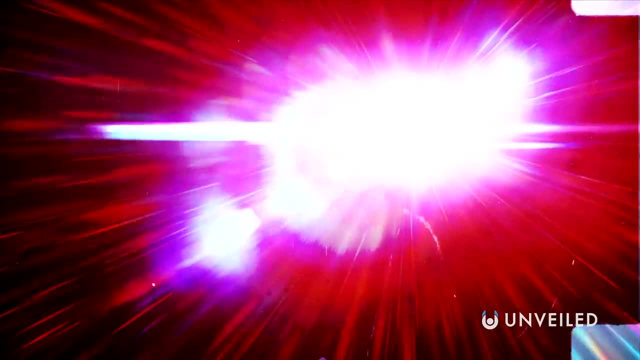 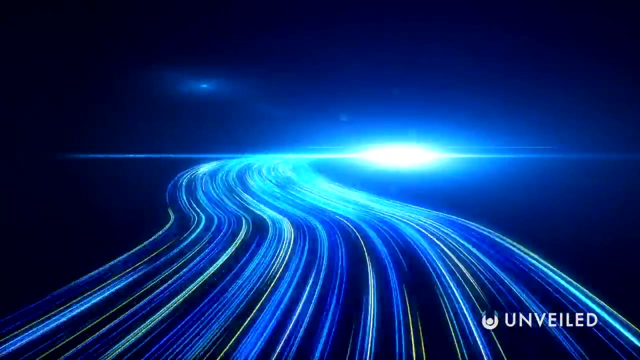 energy cosmic ray ever seen, And though there have since been some similar cosmic rays detected, none have truly come close to matching this one. The OMG particle had around 320 exaelectron volts of energy and was travelling at 99.99% percent the speed of light. 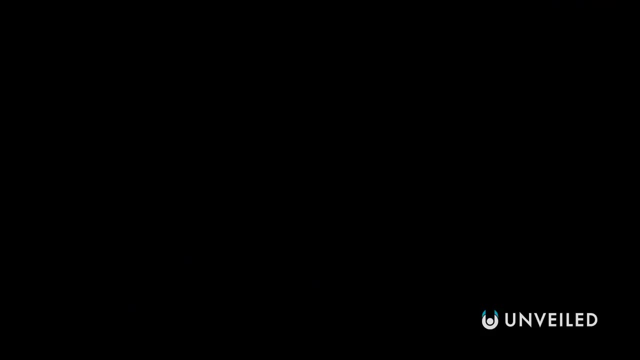 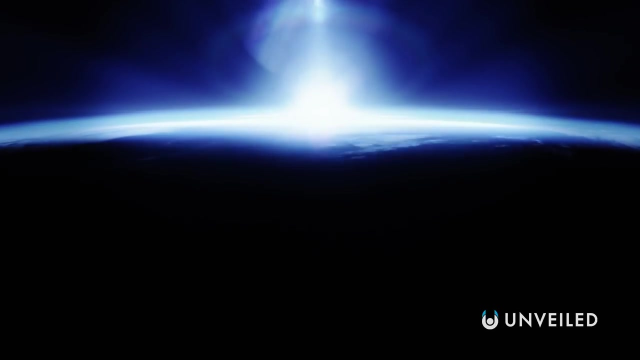 This particular ray was so baffling that the scientists who observed it reportedly held back their discovery for another year before announcing it to the world… because they feared that it had simply been a crazy anomaly. We'd really never seen anything like this before, Even by today's 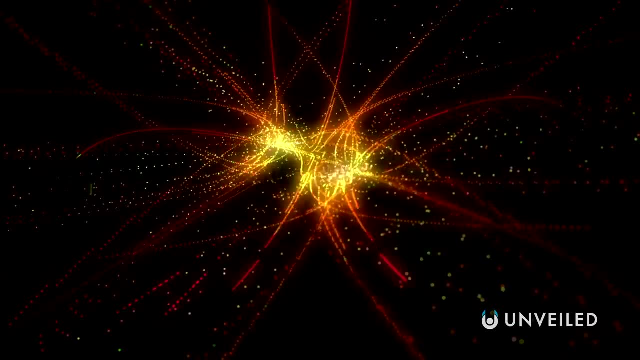 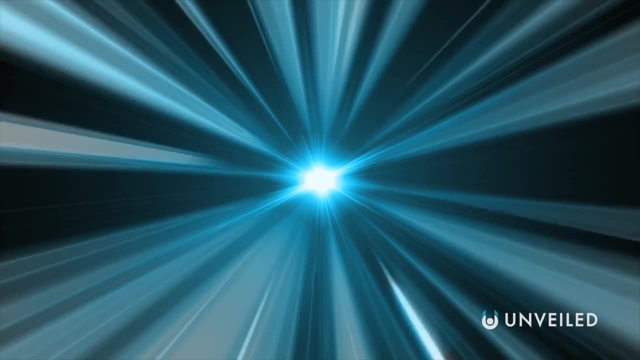 standards, the OMG particle was around ten million times faster than any of the particles we've since accelerated inside the world's largest machine, the Large Hadron Collider. Specifically, the- Oh My God- shattered something called the Grison-Zetsepin-Kuzmin limit, which was named after 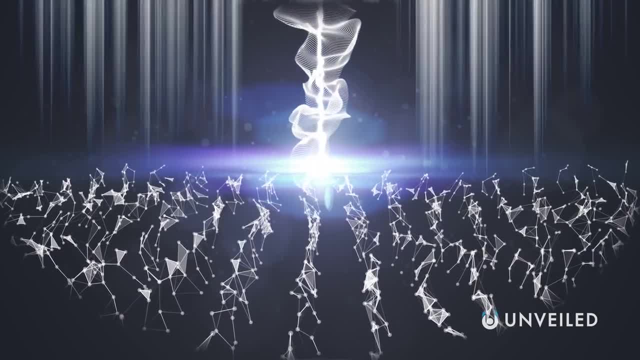 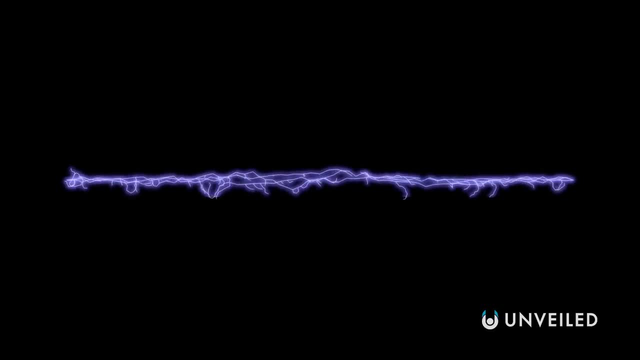 physicists who came up with it and is more commonly called the GZK limit. Formulated in 1966, the GZK limit said that no cosmic ray could ever have energy higher than 60 exaelectron volts. This was because, despite how it appears to us, space isn't just space: It's full of particles. 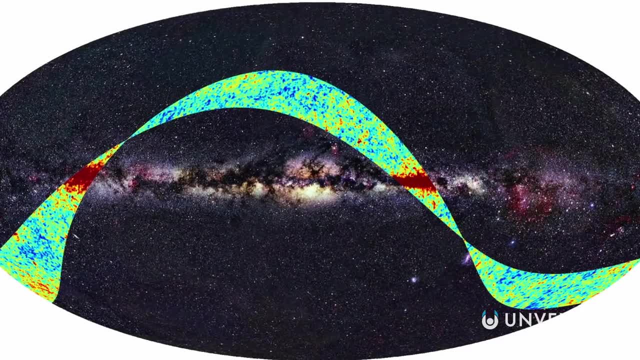 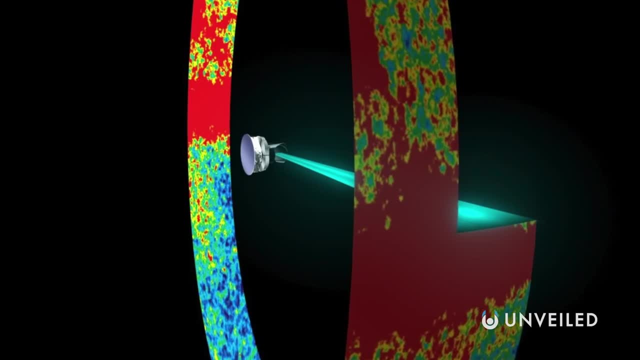 including, and most importantly in this case, the photons that make up the Cosmic Microwave Background Radiation, or CMB. The GZK limit posits that if a cosmic ray had a higher energy than 60 exaelectron volts, the photons would have a higher energy than 60 exaelectron volts. The 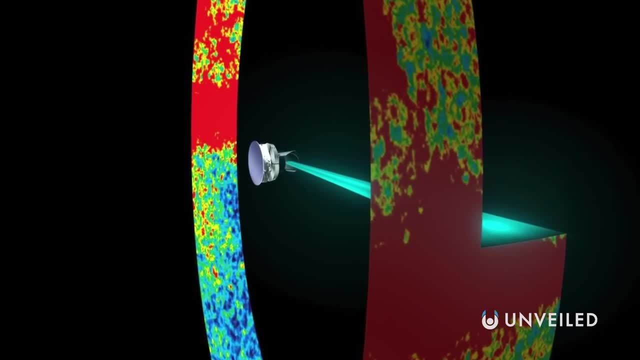 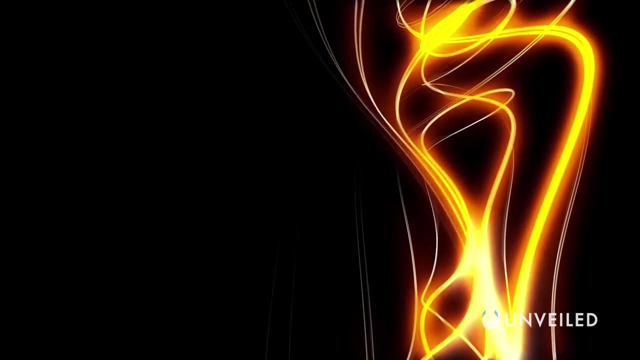 particles in the CMB would effectively stop it in its tracks, with cosmic ray particles crashing into CMB particles. But the OMG particle broke the GZK limit more than five times over and since its discovery there have been a few hundred other extreme energy rays found to have exceeded 60 EEV. 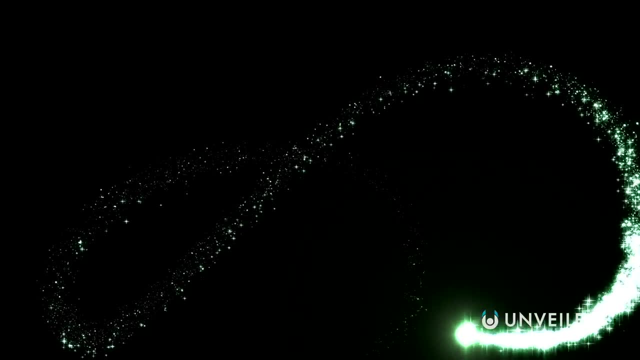 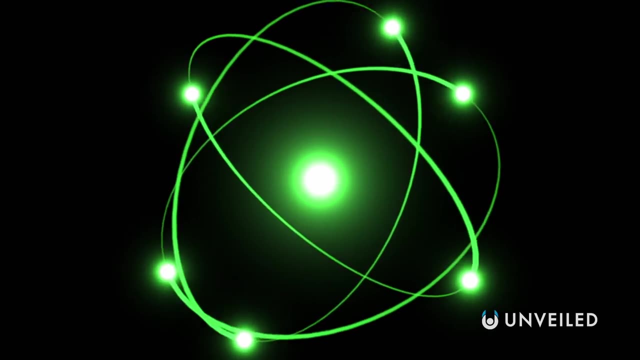 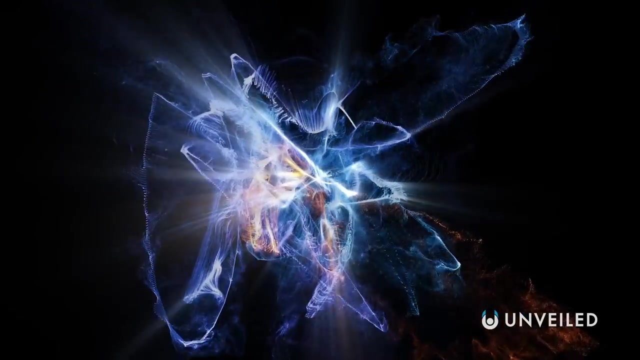 One explanation for violations of the GZK limit has to do with the particles themselves. It's suggested that the GZK limit still applies when the particle in question is a proton, but that the particles in these trans-GZK decay events. the Extreme Energy, Cosmic Rays are made of heavier elements. 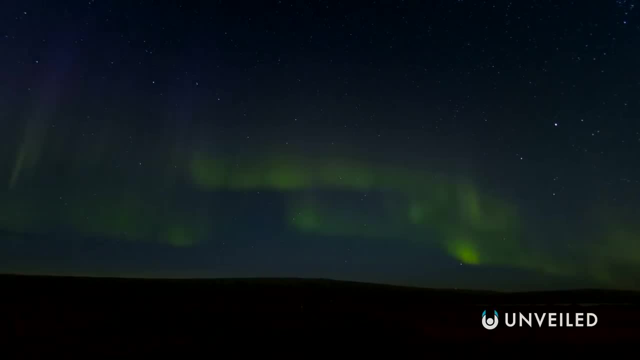 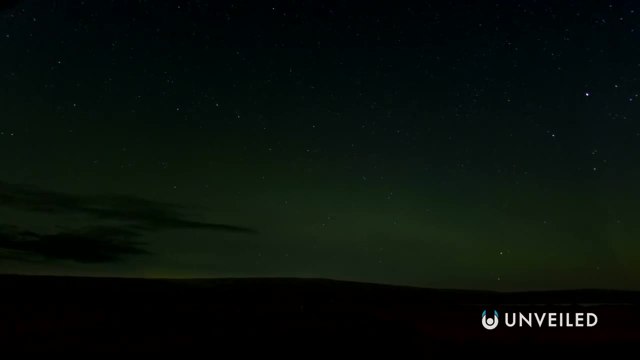 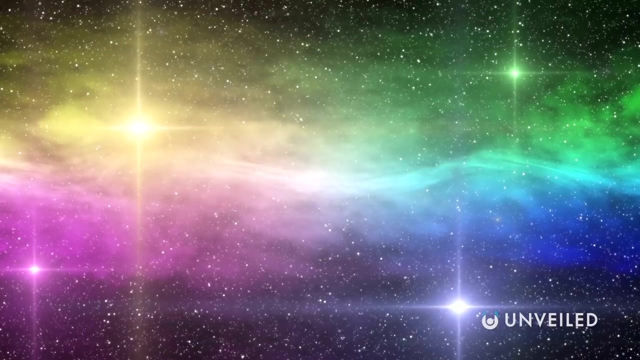 Unfortunately, since it came and went so quickly, we have no way to know now whether the OMG particle was a proton or something else… and it's the same story for all those other Extreme Energy Cosmic Rays detected afterwards as well. For the OMG particle in particular, we also have very little idea about exactly where. 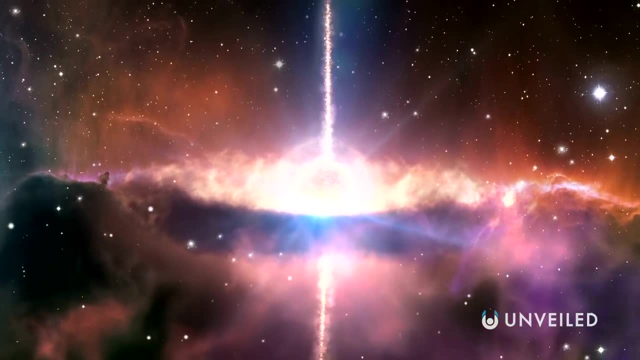 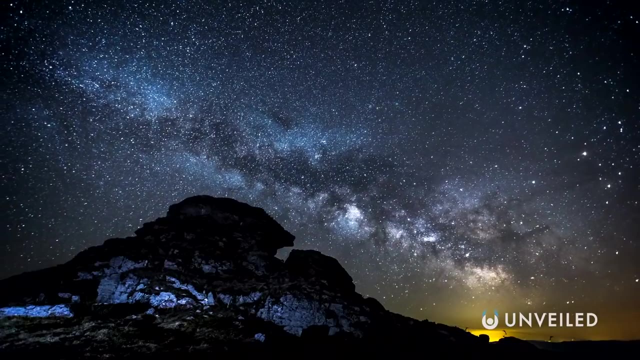 it came from. While it's true that these particles are generally supercharged by incredibly bright objects like quasars or supernovas, when we look into the sky to try and find which quasar or supernova could have launched the OMG particle specifically, scientists are 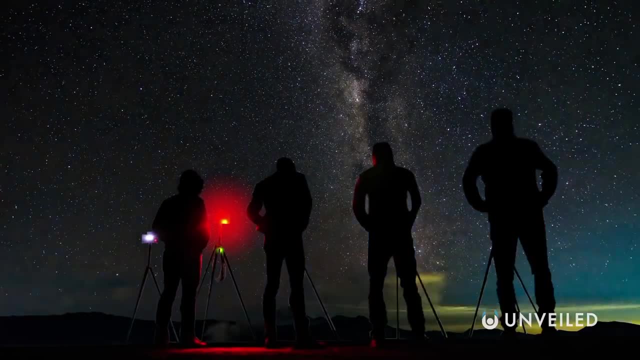 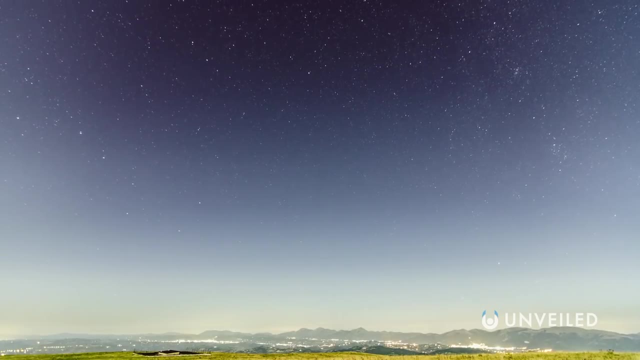 still drawing a blank. One part of the problem is that the trajectory of cosmic rays can be altered by something like the Milky Way's own magnetic field. Observatories have detected that some other cosmic rays appear to come from the vague direction of the constellation Ursa Major, but there's no conclusive path to a source. 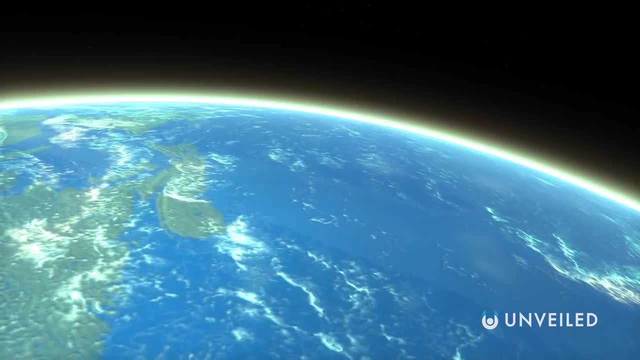 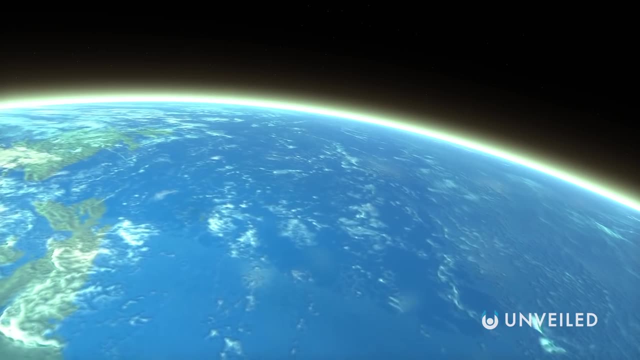 beyond that, Of course. the other main problem when trying to understand cosmic rays of any kind is time. We don't really know about them until they enter Earth's atmosphere, and then it all happens so quickly. We can only see them at all because of Cherenkov radiation, which is the radiation produced. 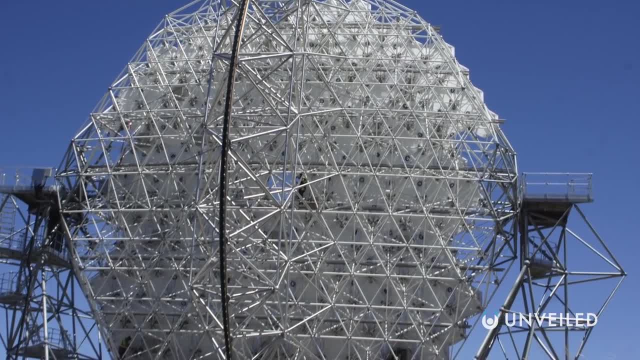 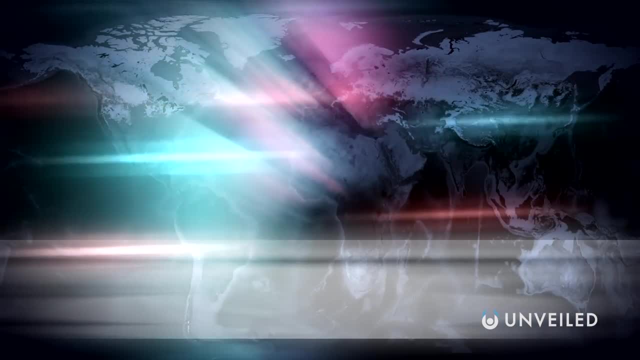 when an object exceeds the speed of light relative to the medium. it's in Water, perhaps, But even then they're only very briefly visible. With the OMG particle, because of the huge amount of energy it harboured, it was almost. 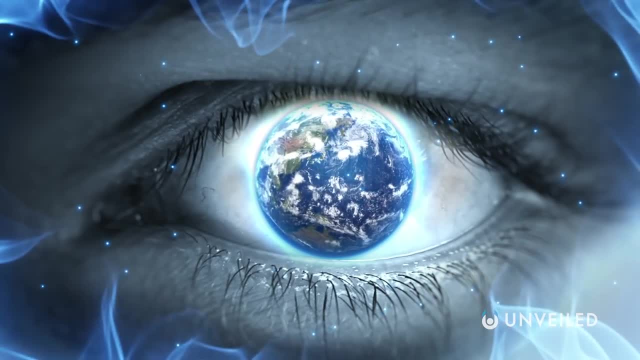 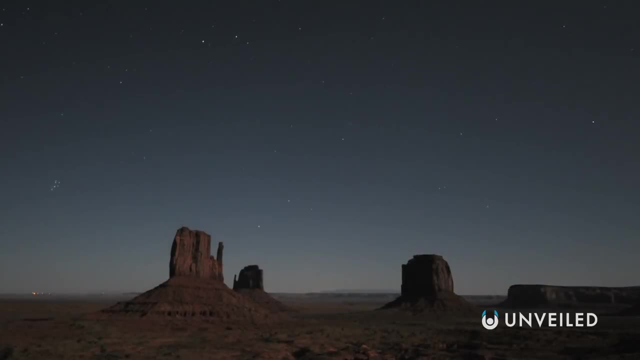 impossible to draw any meaningful conclusions other than… it happened. We are making some progress in studying cosmic rays. However, we don't know exactly how long it will last. The telescope array project in Utah- the same state- the OMG particle was discovered in. 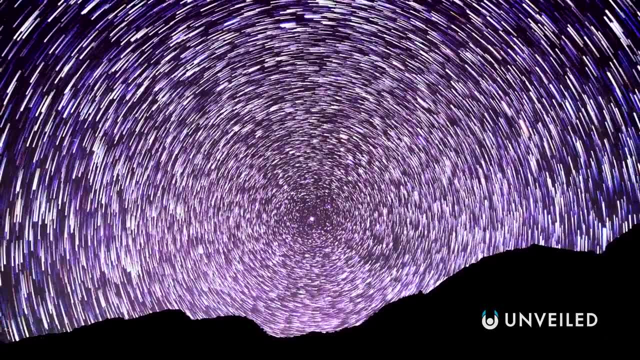 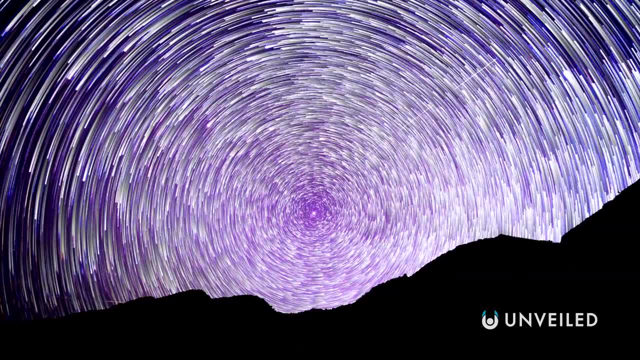 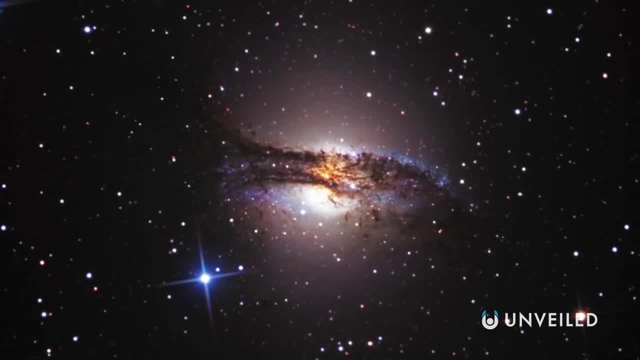 started up in 2008,, with 507 surface detectors. One key finding of the array so far has been that about 27% of all the detected ultra-high energy cosmic rays we experience come from just 6% of the sky. This apparent hotspot once again appears to lie in the direction of Ursa Major, so we 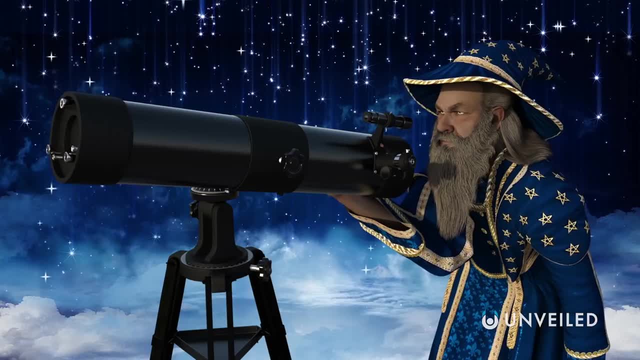 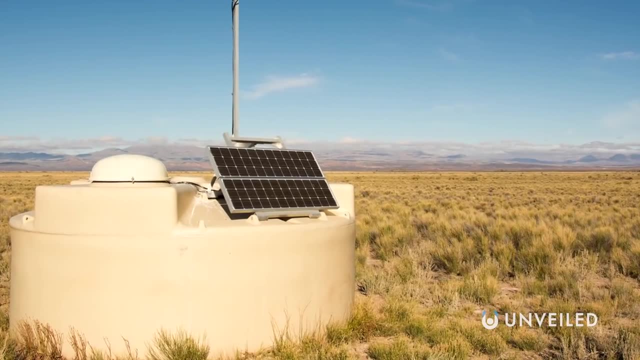 are at least searching in roughly the right place, But there are still many more puzzles to solve, Especially as the Pierre Auger Observatory in Argentina has reportedly found evidence of another warm spot in the direction of Centaurus A, the fifth-brightest galaxy in.